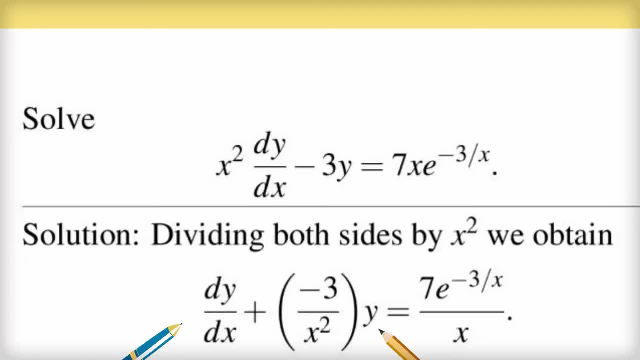 square root of y. We can't have cos y, anything like that. So this equation satisfies that requirement that both dy, dx and y just appear as they are. I don't have any powers or anything like that. The next thing is, though, we can have an. 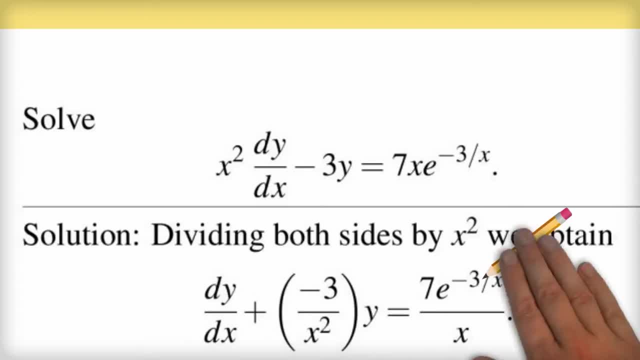 expression or a function of x in front of the y. So here I've got minus 3 divided by x squared, but here we could have any function in x that we like: cos x, x divided by 1 plus x squared, Whatever you like. And similarly over on the right hand side we can have any. 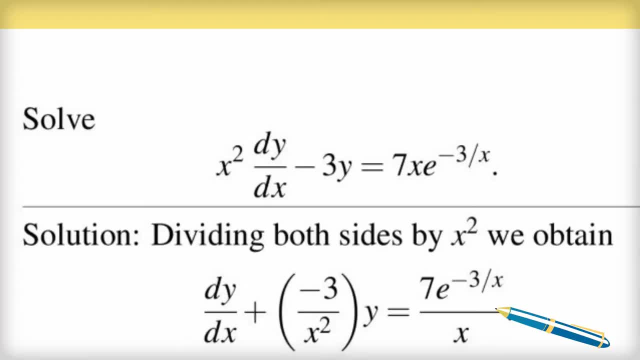 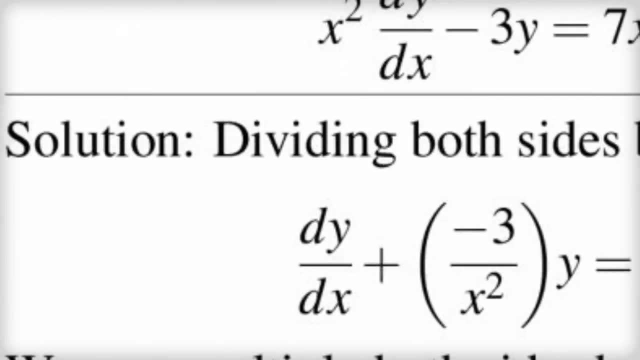 equation in x that we want as well. So that's that. That's the answer to the question. I'm wrong or wrong was the answer to the remaining, So let's just take a moment to preview how this works, because it's very clever. 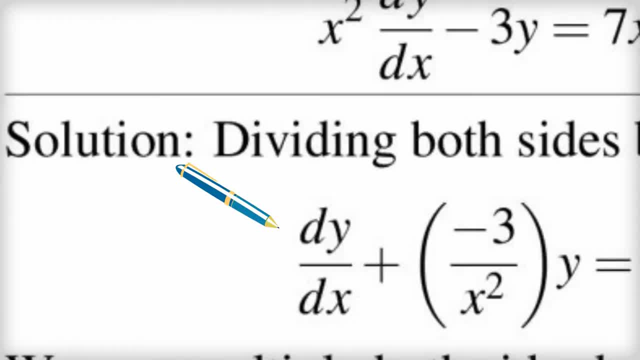 Someone looked at this and they said, look, what we've got on the left-hand side is sort of the beginnings of the product rule for differentiation. So, for example, if I take the derivative of, say, y times sine x, well, I get dy dx by sine. 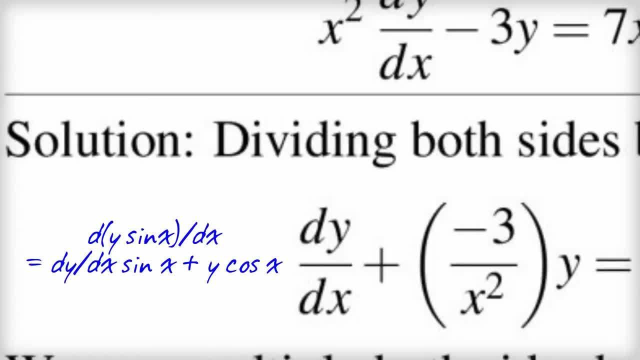 x plus y times cos x. So I've got this sort of dy dx and I've got a y and you can see, here I've got the beginnings of that. here I've got a dy dx term and I've got a y term. 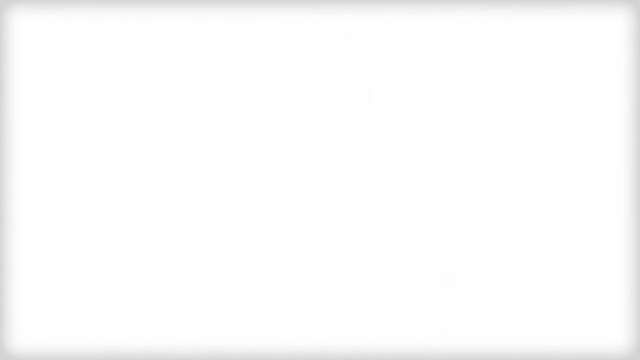 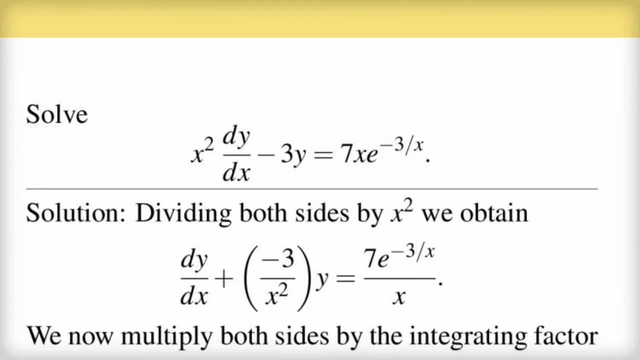 So someone worked out- someone cleverer than me worked out- precisely what needs to be multiplied by both sides by, so that we actually get the results of the product rule, In other words, so that we can then crystallize the left-hand side. 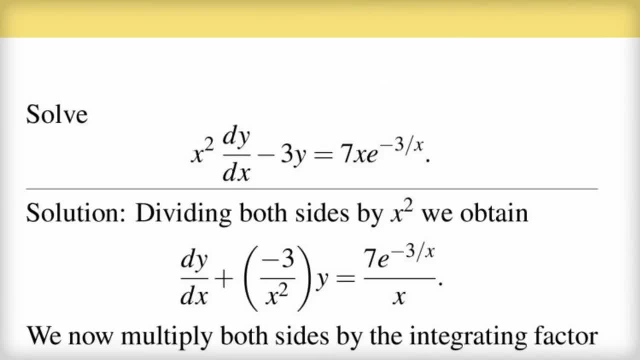 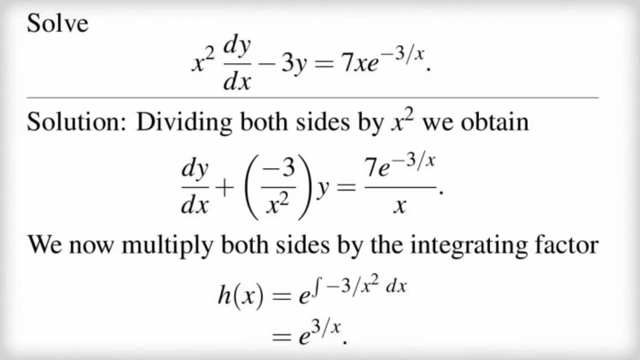 Or shorten the left-hand side by using the product rule in reverse. So here's how we work out what to multiply both sides by. It's called the integrating factor, which I've called hx, And the way we do that is we take e, we take to the power of the integral of, and then 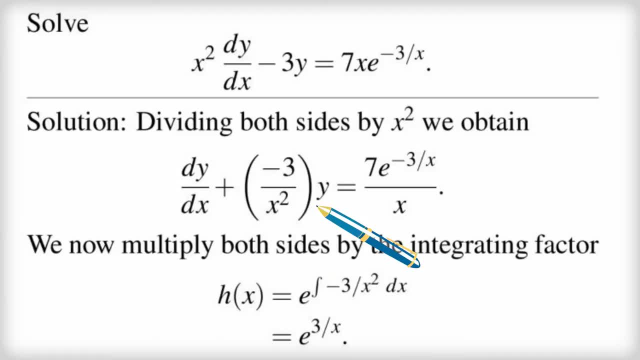 we put in whatever we've multiplied y by in our equation. So in my case here I've got negative three divided by x squared. So I put that in the integral, I do the integration And I'm left with hx. equals e to the power of three divided by x.